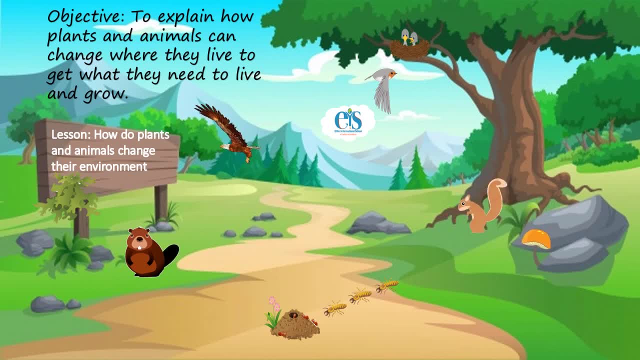 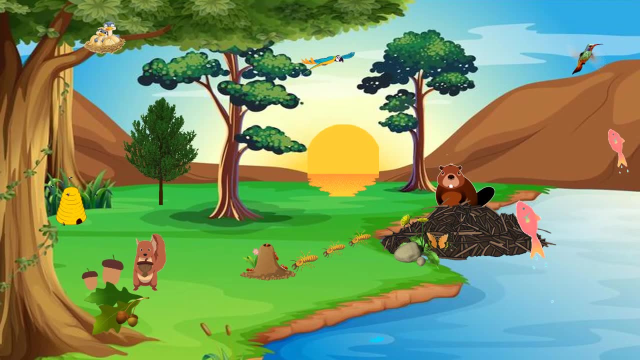 So are you ready to learn more about our lesson? Okay, let's get started. Let's begin our lesson by learning about how do animals change their environment. So let's take a look at this scene and name the animals we see. So here we have birds in a nest, some bees, a squirrel holding its acorn. 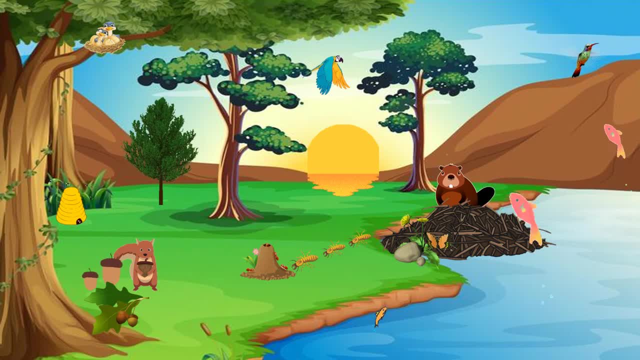 some termites, a butterfly, some fish, a beaver, a parrot and a hummingbird. So how do some of these animals change their environment? First, let's begin with this brown animal which is called a beaver. 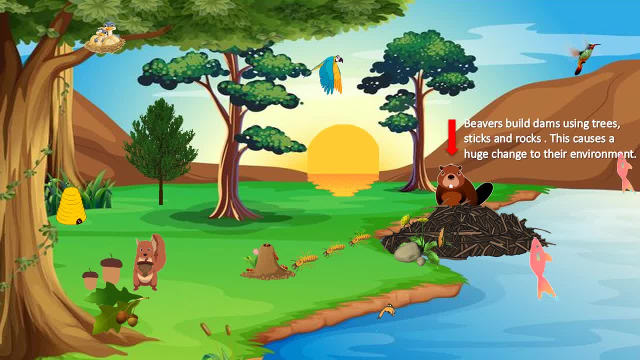 Beavers build dams. They sing trees, sticks and rocks, And this causes a huge change to their environment. What about squirrels? How do they change their environment? Squirrels bury nuts under the ground And sometimes they forget where did they bury these nuts? 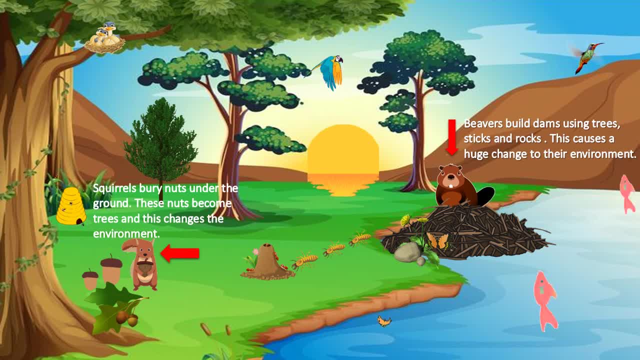 So these forgotten nuts become trees, and this changes the environment. Now, what can we see next to the squirrels? Yes, these are called termites. Termites change the environment by using soil to build their mounds, And this returns back minerals to the soil. 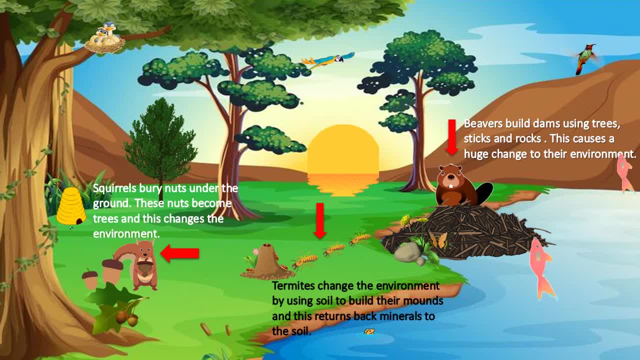 What are these animals flying above the beehive? They fly above the beehive. What are these animals flying above the beehive? What are these animals flying above the beehive? What are these animals flying above the beehive? 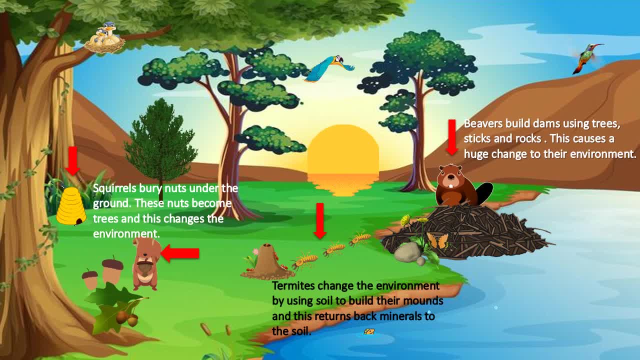 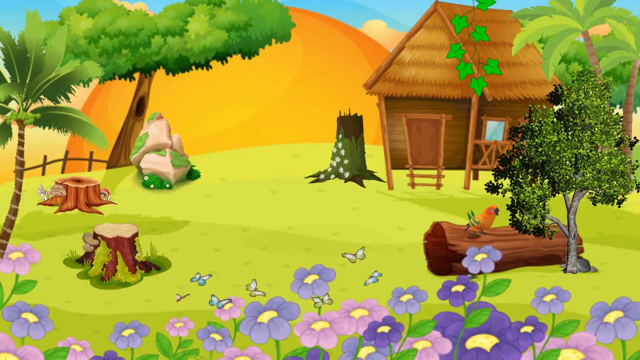 What do we call them? Very good, These are called bees. Bees also change the environment by transferring pollen between flowers, And this helps flowers grow, breed and produce food. And this helps flowers grow, breed and produce food. What about plants? 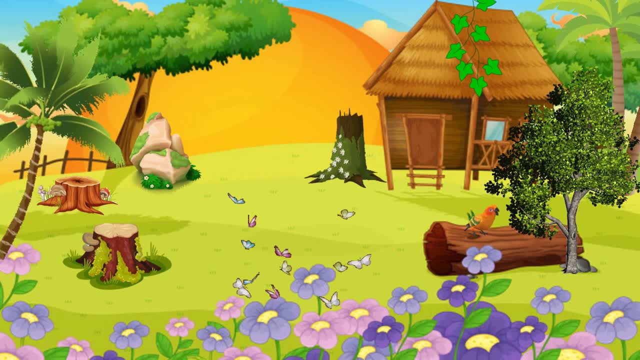 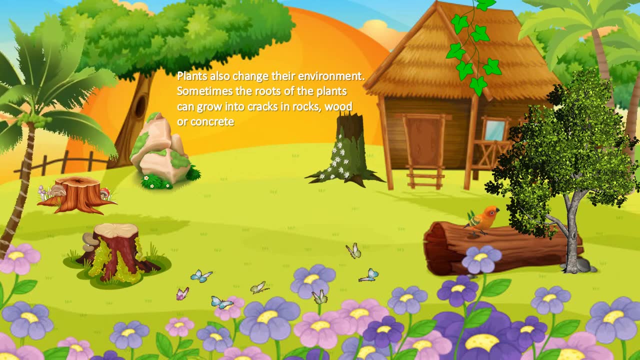 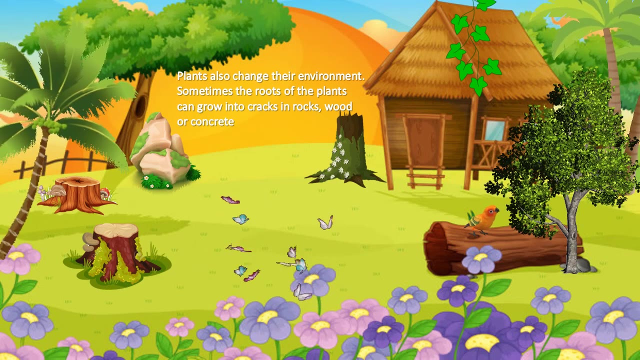 What about plants? What about plants And how can plants change their environment? Well, plants can change their environment, where sometimes the roots of the plants can grow into cracks in rocks, wood or concrete. So take a look at this beautiful scene and tell me. 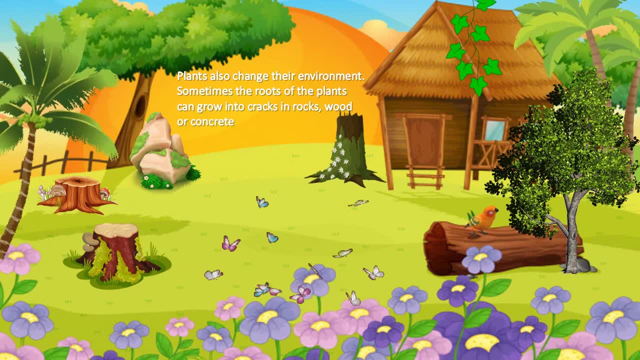 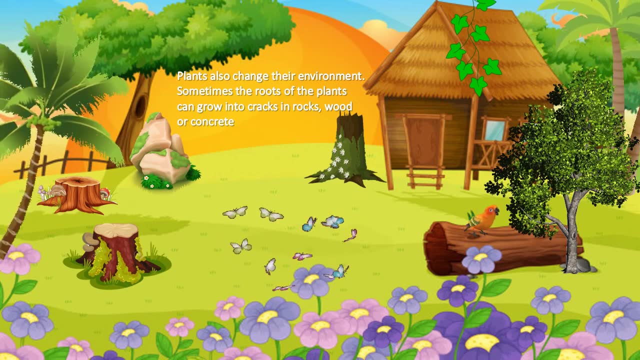 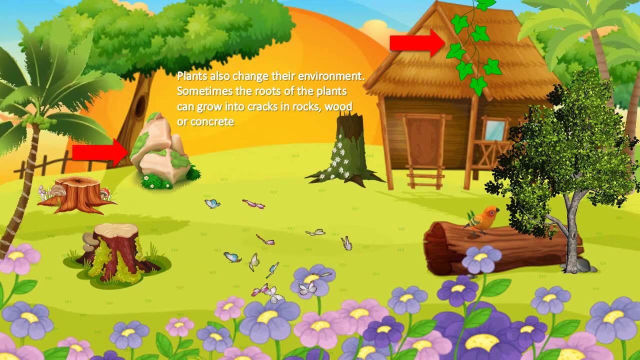 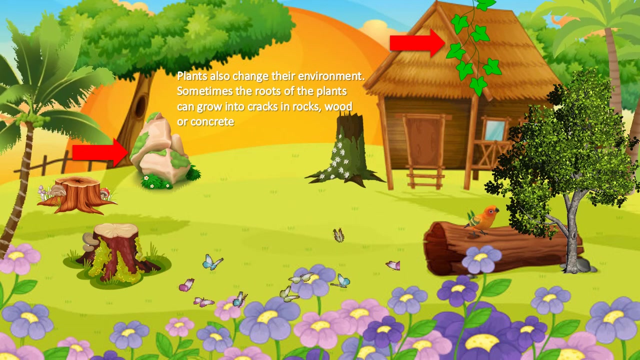 Can you see examples of plants changing their environment? Can you see examples of plants changing their environment? Fantastic job. Yes, we do. We can see a plant called ivy, which is a kind of a climbing plant that grows on houses. We can also see plants that is growing into cracks in rocks and in wood. 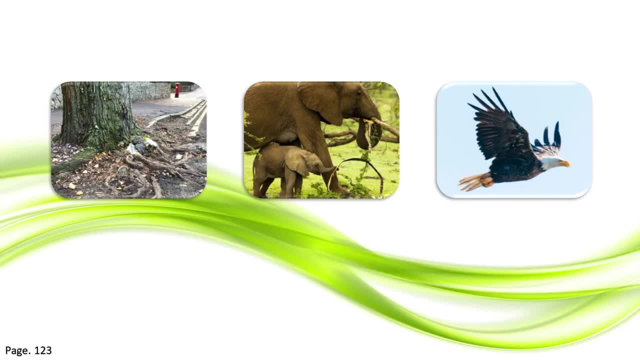 Well done. And now let's open page 123 in our science book, where we are asked to circle the pictures that show plants or animals changing their environment to get what they need. So which pictures are we going to circle? Very good, We are going to circle the picture of the tree. 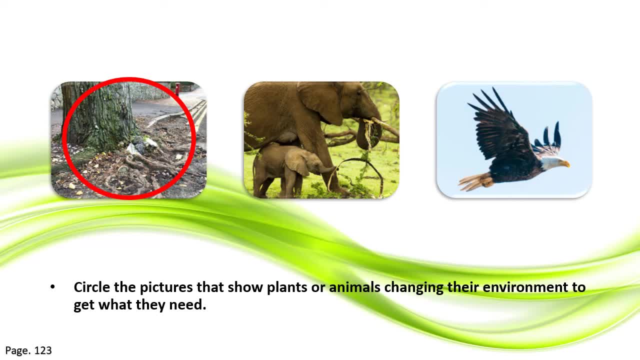 where we can see that the tree roots pushed and broke. The tree roots broke the concrete, which caused a change in the sidewalk and the street We are also going to circle the picture of the elephants And in this picture we can see that the elephant is using his long trunk to wrap around small twigs and branches. 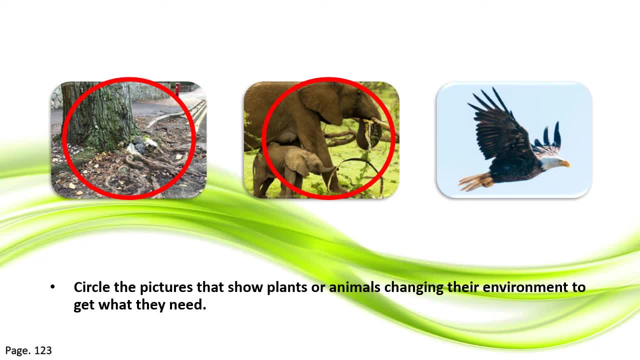 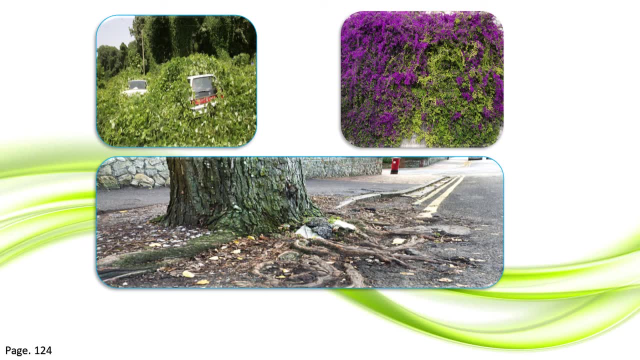 to break them off and bring them to his mouth. Well done, Let's see the picture of the elephant. Let's move on to page 124 in our science book, where we are asked to circle the parts of the environment that changed. So, first of all, we are going to circle the picture of this beautiful purple flower. 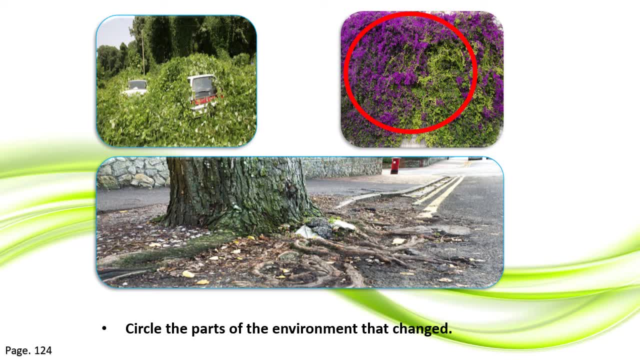 This flower needed a lot of space to grow and that's why it grew over a wall. We are also going to circle the picture of the car. We are also going to circle the picture of the car. These plants used the car to get enough space to live and grow. 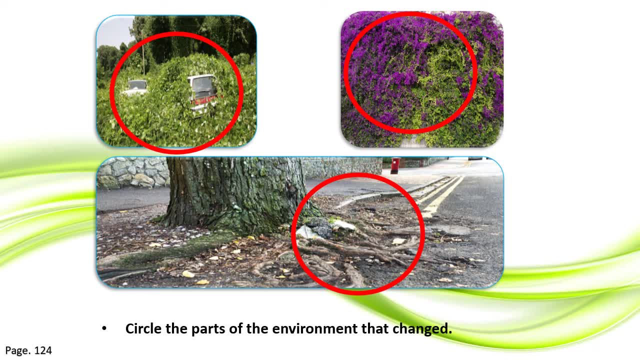 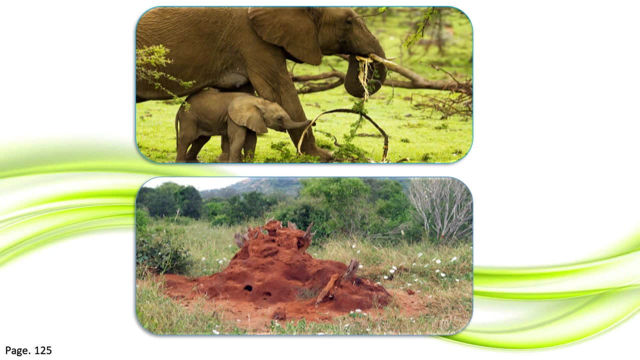 And last of all, we are going to circle the roots of the tree. in the third picture, This tree caused a change in the sidewalk and the street because the tree roots have pushed and broke the concrete. moving on to page 125 in our science book, where we are asked to circle the parts of the environment, 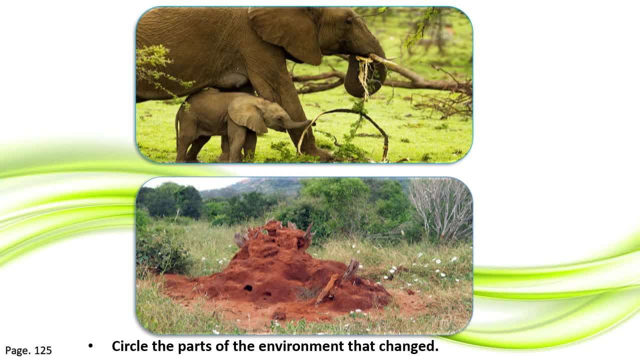 that changed. so what do you think? good job. we are going to circle the picture of small twigs and branches in the elephant's mouth. as said earlier, the elephant uses his long trunk to wrap around small twigs and branches, to break them off and bring them to his mouth. we are also going to circle the picture of 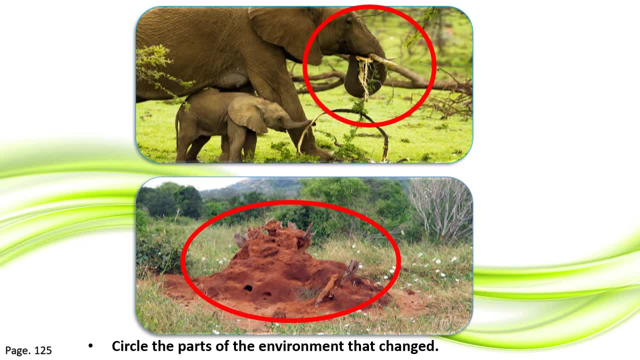 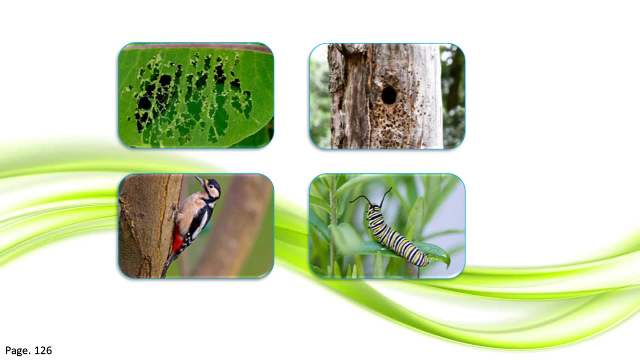 the mound below. termites change their environment by moving on to page 125: moving the soil. the termites move the soil to build the mound. the mound is their shelter. now let's open page 126 in our science book, where we have four pictures of a leaf with holes in it. 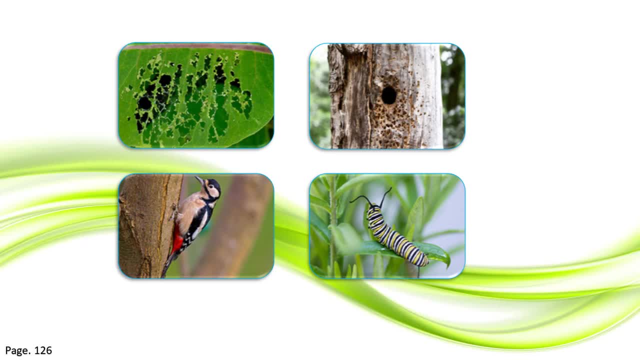 a bark of a tree, a woodpecker and the caterpillar. and here we are asked to draw a line from the animal to the environment. it changed. so first of all we have to draw a line from the caterpillar to the leaf with holes in it. did you know that caterpillars eat leaves? 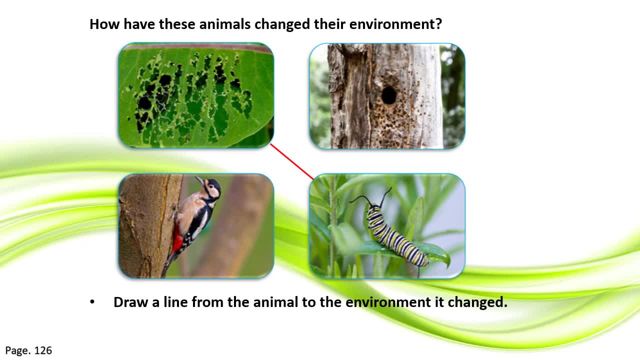 so the caterpillar changes its environment. the caterpillar ate the leaf above, and now the leaf has holes in it. what about the woodpecker? how does it change its environment? well, woodpeckers eat insects that live under the bark of many trees. so here we have to draw a line from the woodpecker to the bark of the